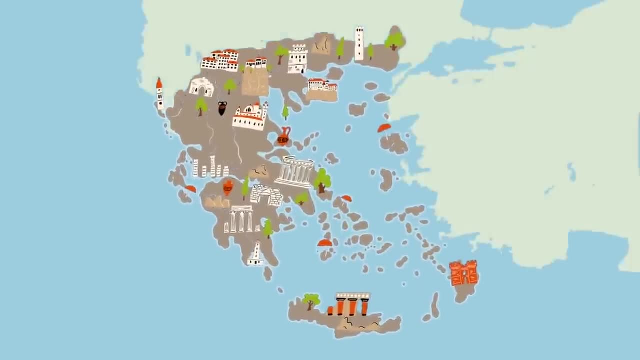 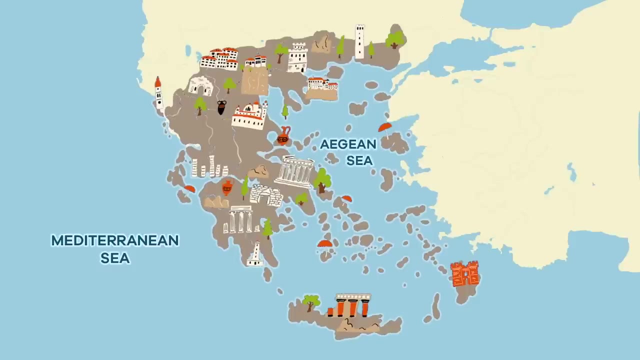 Ancient Greece was found in what is now called Southeastern Europe, along the coast of the Mediterranean Sea on the west and the Aegean Sea on the south. On the east, right across from modern-day Turkey. About 80% of the land was full of mountains, which provided the people with natural barriers. 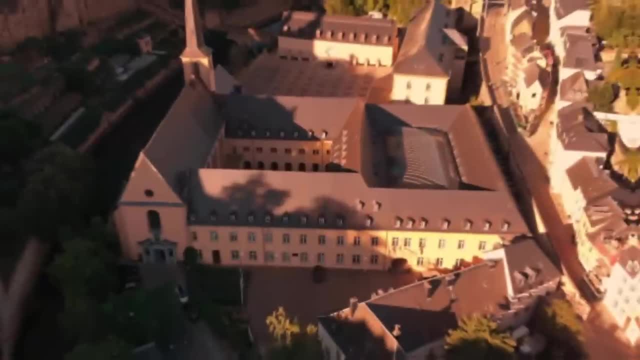 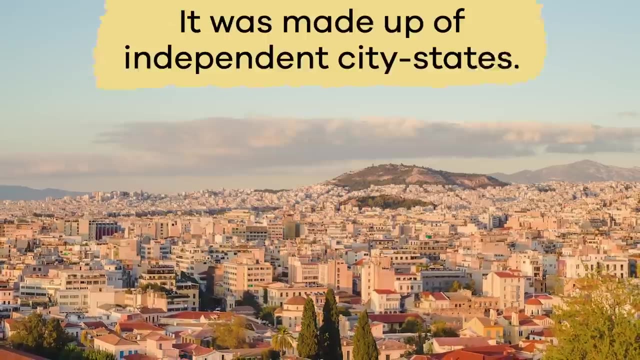 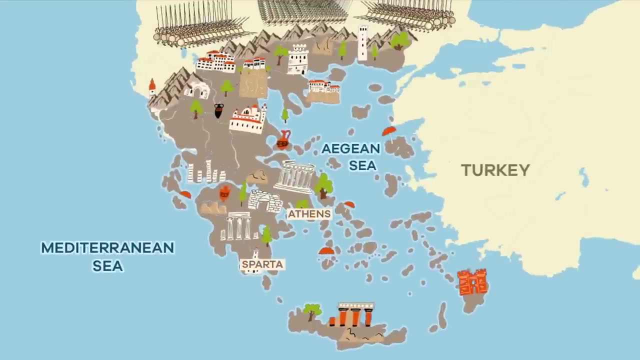 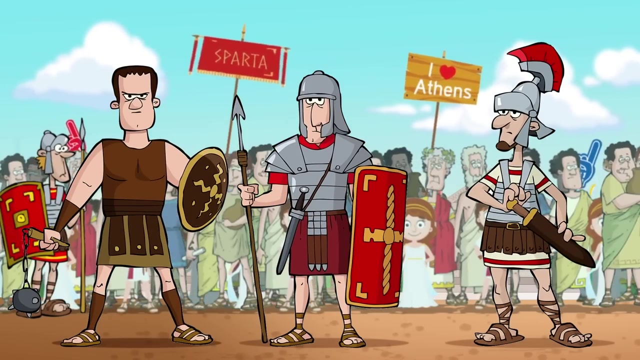 of protection from potential enemies. Unlike modern kingdoms or countries today, Ancient Greece was not one large empire. Instead, it was made up of various independent city-states, including Athens, Sparta and Greece, Even though these city-states were separate from each other and often fought or competed. 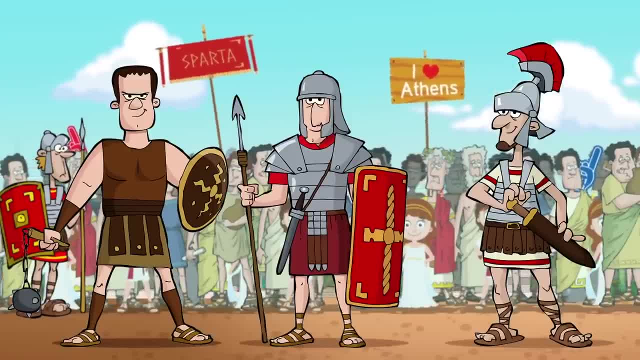 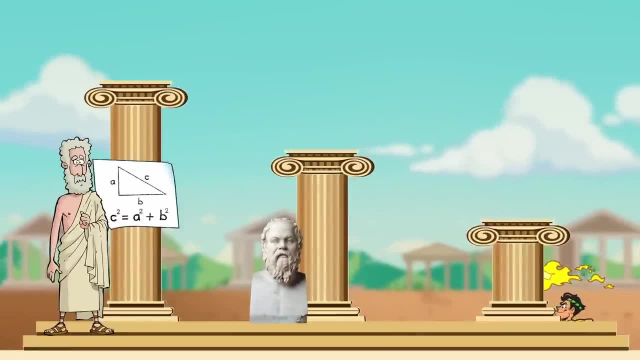 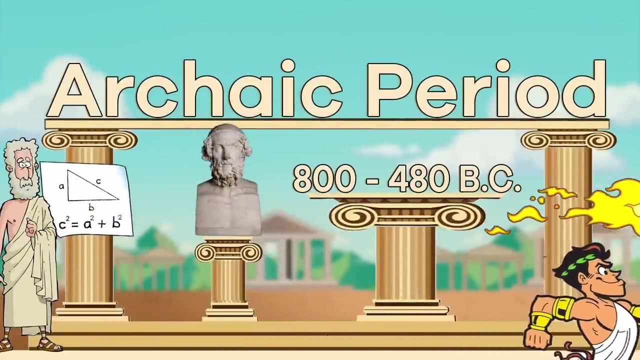 against each other. they all spoke the same language and had similar cultures and customs. Much like other great civilizations, Ancient Greece was divided up into time periods, each one with its own unique events and contributions. First is the Archaic Period. The Archaic Period is the period of the period between 800 and 480 BC. 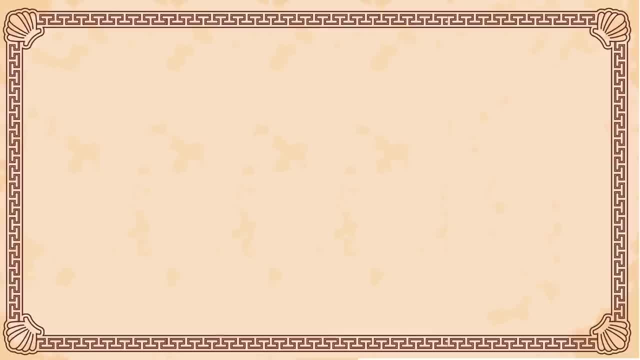 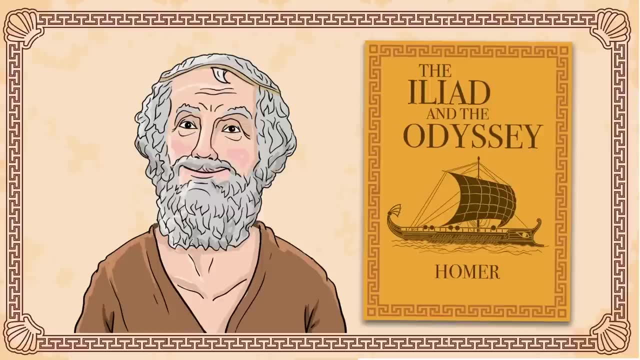 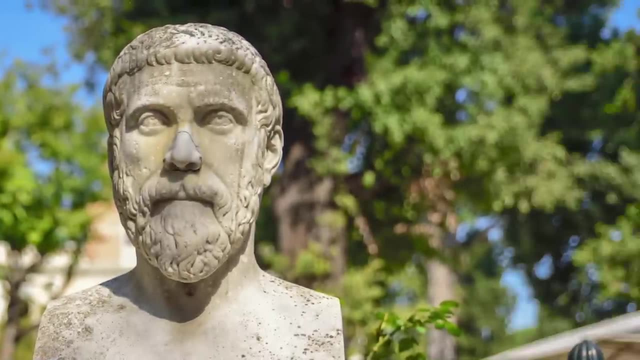 The first Olympics was held during this time and the philosopher and writer Homer wrote two of the most famous poems in the world's history, Iliad and Odyssey. And a famous mathematician and scientist named Pythagoras was born. We still use his Pythagorean theorem. 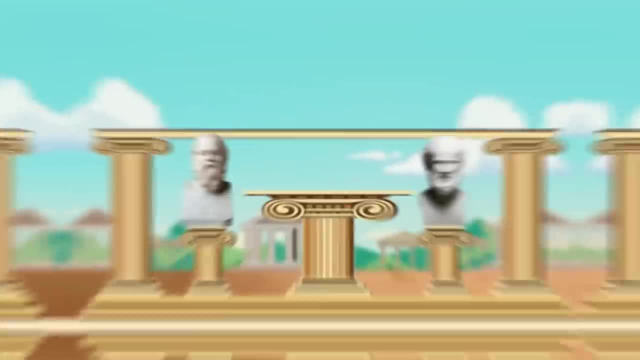 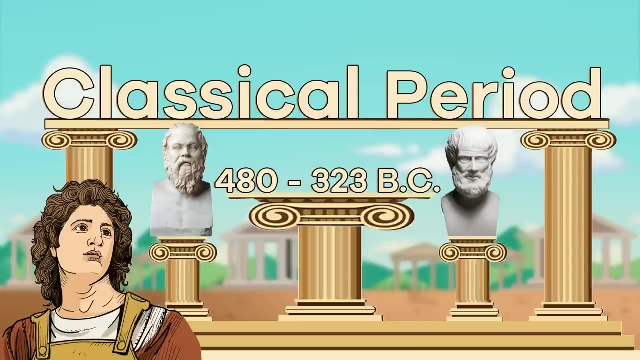 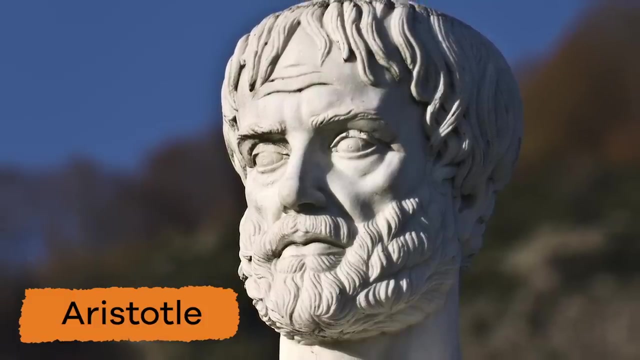 In general, the Pythagorean theorem is correct. For example, the Pythagorean theorem is a very common and common practice Geometry Today. Next is the Classical Period, which lasted from 480 BC to 323 BC. The famous philosophers Socrates and Aristotle lived during this time. Alexander, the Great ancient Greece's most famous leader, was also born and eventually conquered many lands surrounding the Greek Empire after he became king And the Parthenon, which is a temple in honor of the goddess Athena, was built in the city-state. 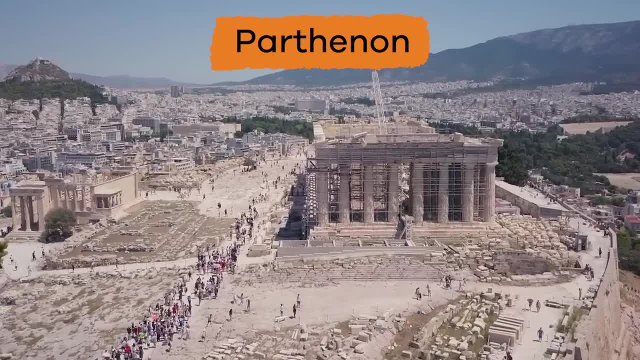 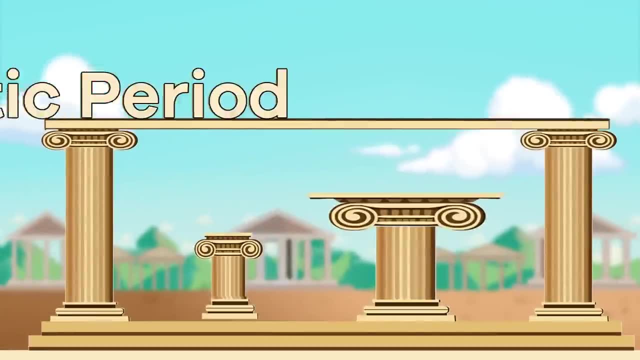 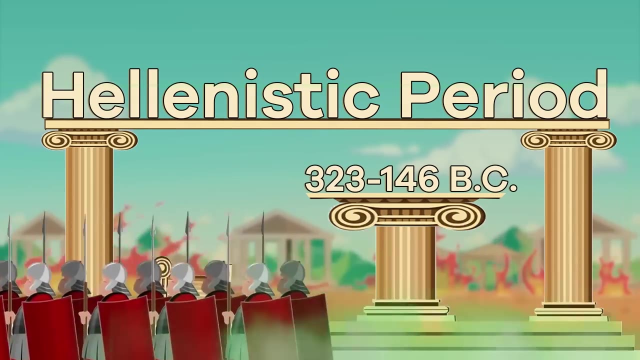 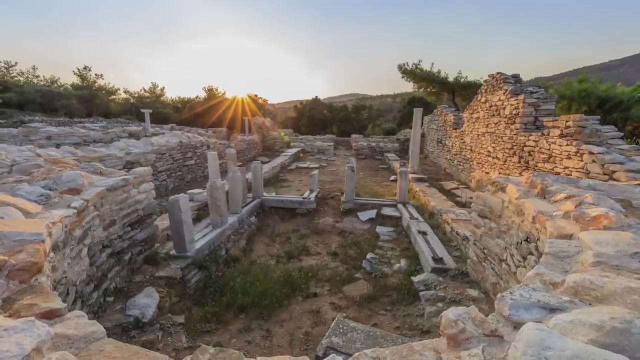 of Athens, The Parthenon still stands today and is the oldest ancient Greek building to survive in modern times. Last is the Hellenistic Period, which spanned from 323 BC to 124 BC. This era marked the death of Alexander the Great and the decline of the ancient Greek. 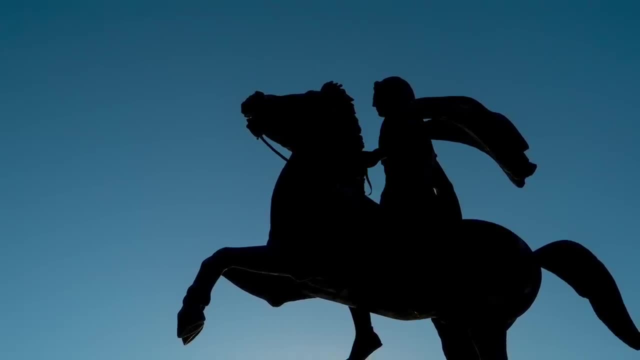 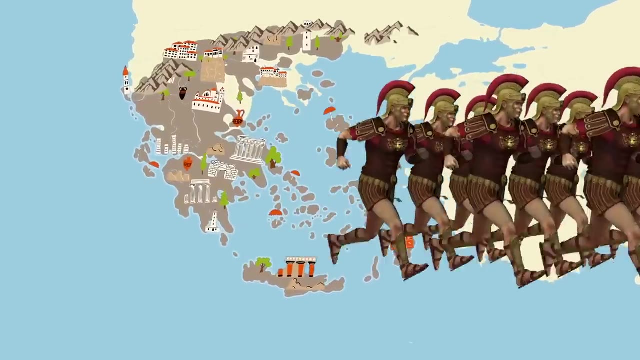 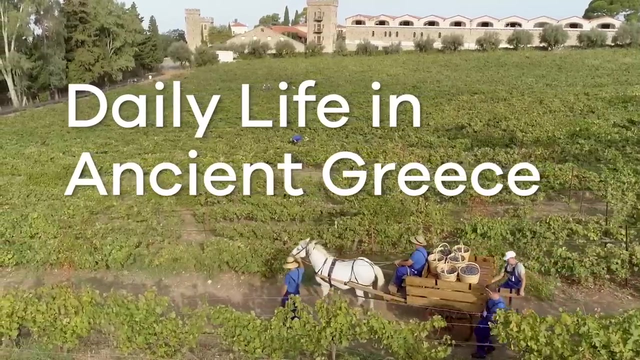 civilization. After Alexander the Great died, the ancient Romans began to conquer Greek lands, eventually making all of ancient Greece a part of the Roman Empire. Now let's explore a little bit about what daily life was like. The rooms of Greek homes were built on the walls. 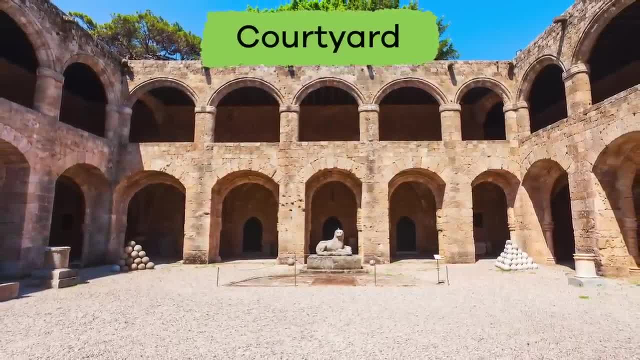 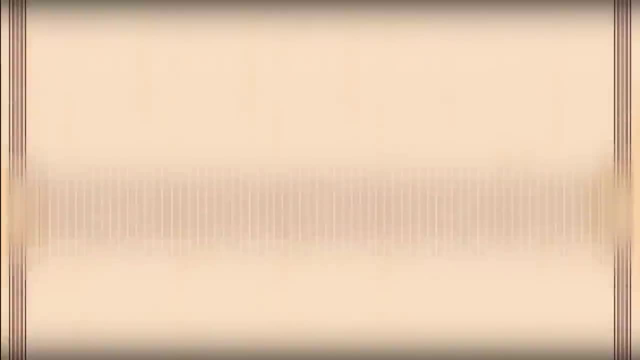 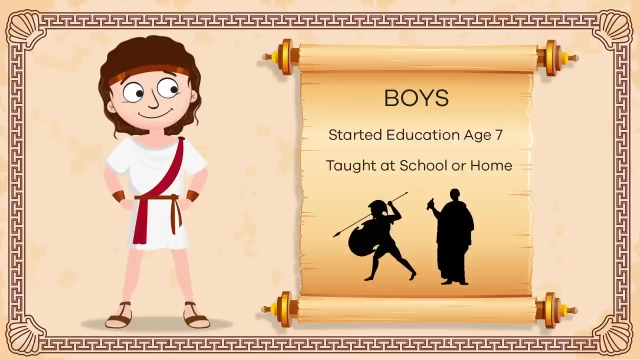 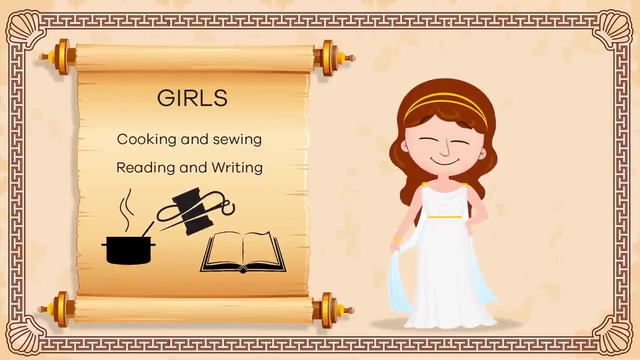 water and an altar for religious worship. Children were treated differently based on their gender, Depending on the city-state. boys were formally educated starting at age seven, either at school or at home. Girls, on the other hand, learned homemaking skills like cooking or sewing. 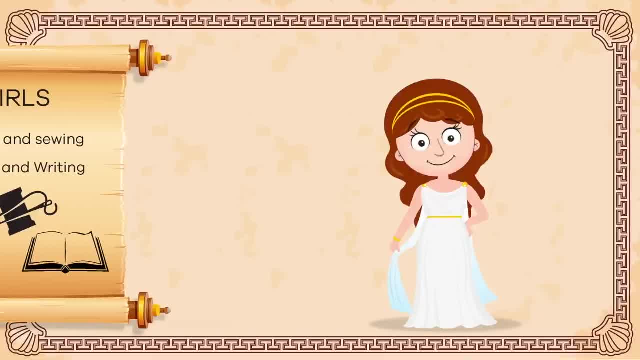 Girls learning homemaking skills could be: 1. て was read and 2. て was read for children. 3. て was being taught genesis and multiplication. This is one way of teaching the book of war to children. 4. girls in the city-state of Sparta received the most education. 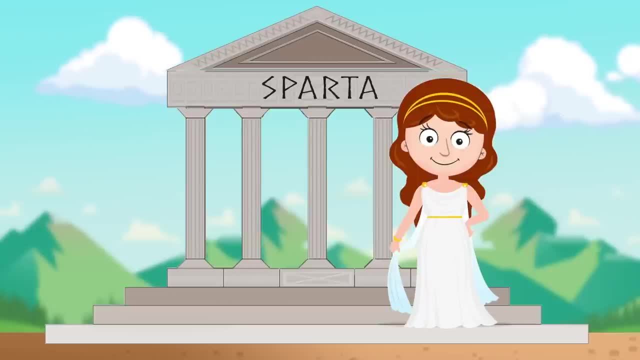 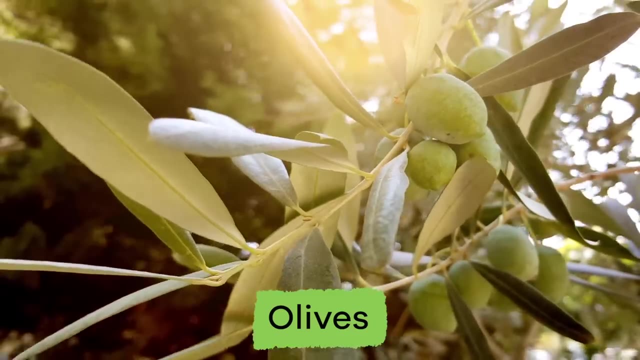 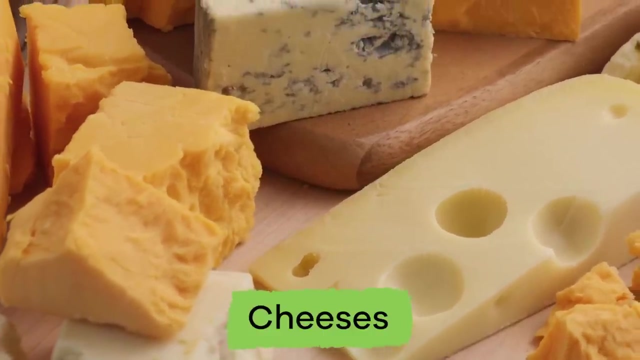 and freedoms of all the city-states in ancient Greece. Most Greek men were farmers, so they ate what they grew. Olives were a very important part of the people's diets. The majority of the Greek diet consisted of Five. Diana the¡­ recorded the official date of the day in the BC ate'­l The%. 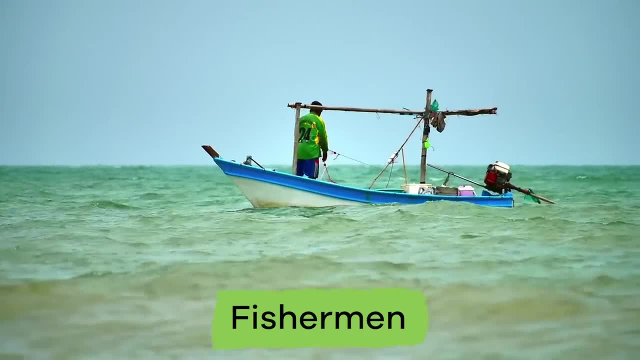 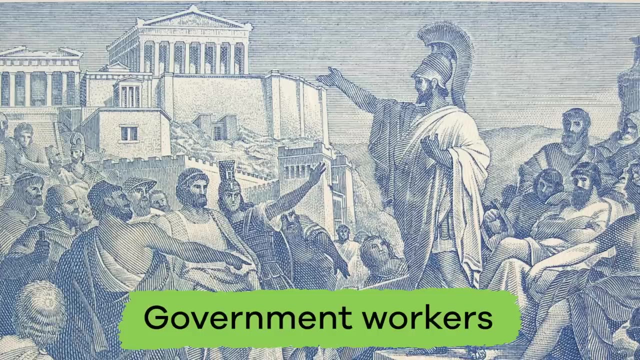 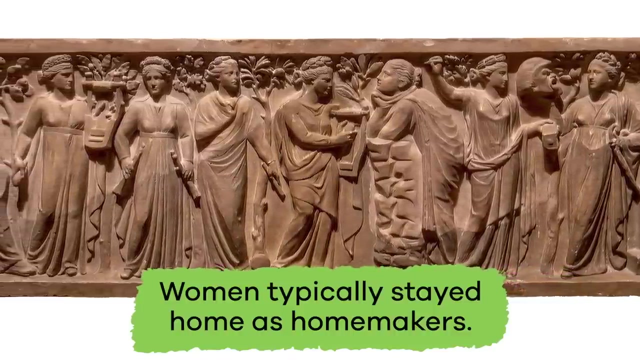 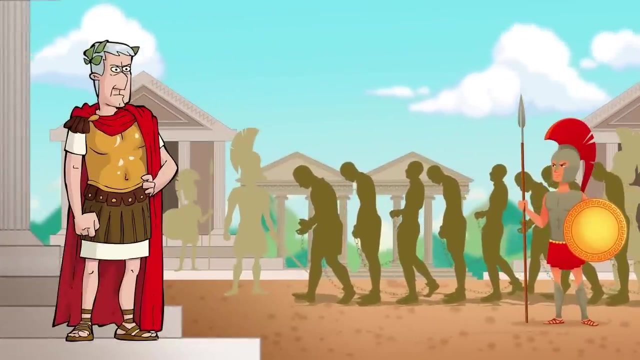 and fish. Other occupations for men included fishermen, soldiers, teachers, government workers or craftsmen. Women typically stayed home as homemakers, caring for children, cooking, sewing and doing other work inside the home. Unfortunately, most citizens of ancient Greece enslaved other people, usually from lands. 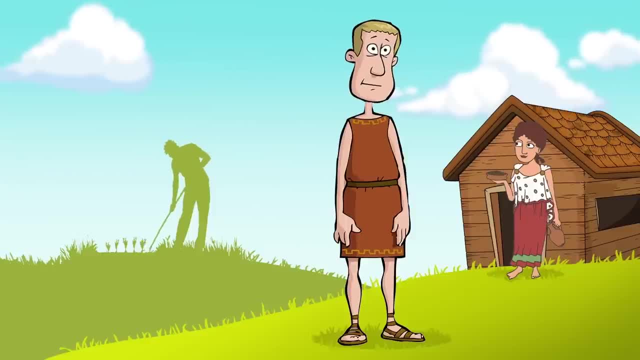 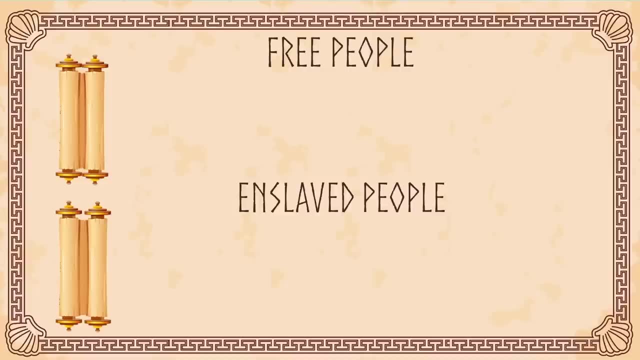 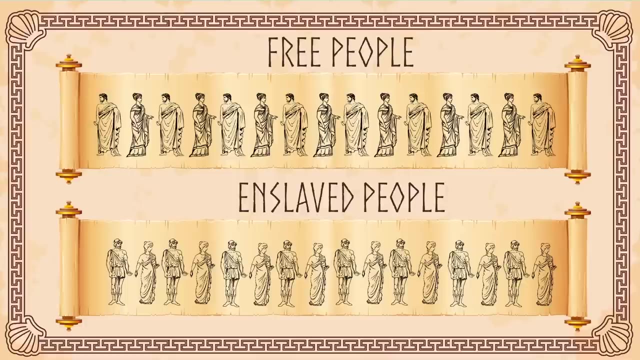 that the empire had conquered. Even the poorest of Greek families typically relied on the labor of at least one enslaved person. In fact, there were about as many enslaved people in Greece as there were free people. So even though the ancient Greeks were advanced in many ways,